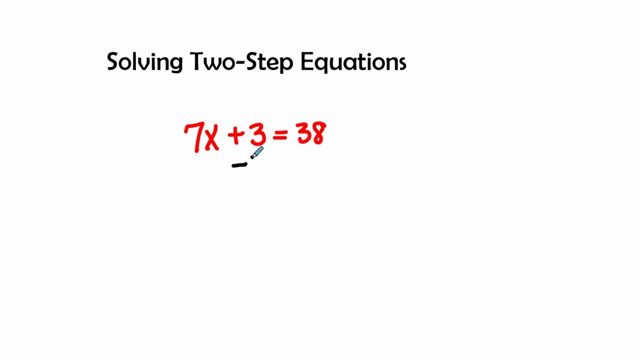 I'm going to take its inverse operation, And so the inverse operation is a negative 3.. So I'm going to move the negative 3.. And what I do on one side of the equation or the left side of the equation I need to do to the right side of the equation. 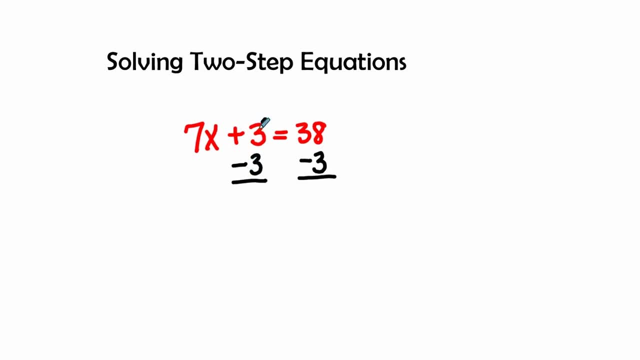 So a positive 3 minus 3 is 0.. And then 38 minus 3 would be 35.. 35.. I'm going to go ahead and bring down my 7x Now I have: 7x equals 35.. 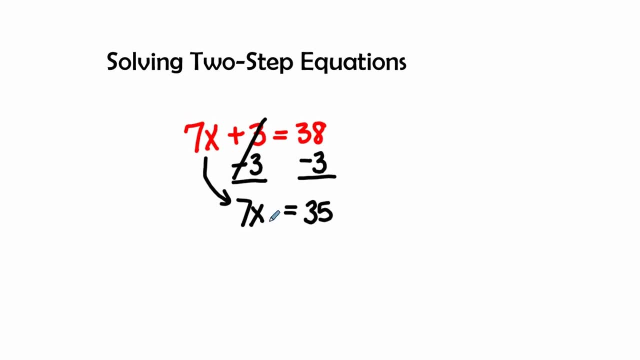 The x is still not by itself, so I need to see how is the 7 attached? Well, the 7 is attached by 7 times x, And with the 7 times x the inverse operation is division. So I'm going to divide both sides by 7.. 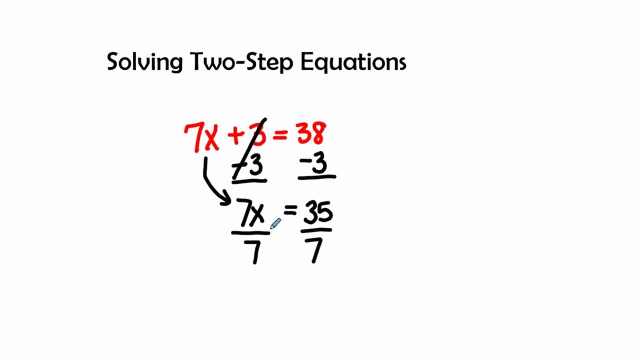 Right there Now. 7 divided by 7 is 1, which leaves me x by itself, with 1x equals. And then I look at 35 divided by 7 is 5.. Now the main thing that I want to look for is how do I check my work? 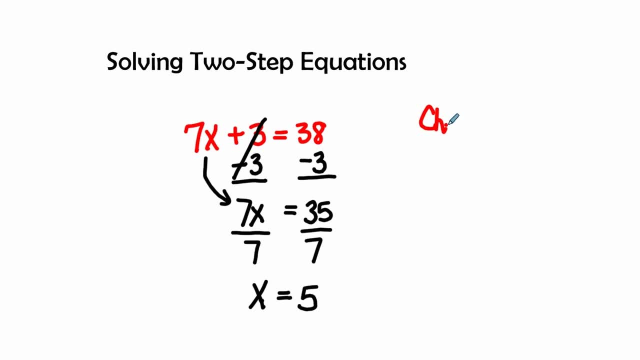 And so over to my right-hand side. I'm going to check to make sure that everything, everything is right on track. So I take my 7, open parentheses, where my variable x, and where I'm going to plug in the 5 plus 3, equals 38.. 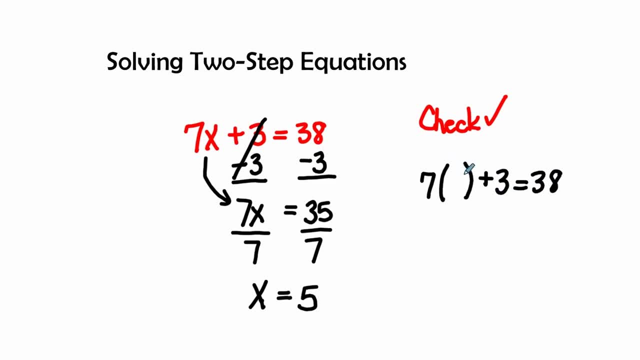 When I plug in the 5,, I see that 7 times 5 is 35 plus 3 equals 38.. 35 plus 3, 38 equals 38. Therefore, I know that my equation is correct. Just as a reminder when we are solving two-step equations: